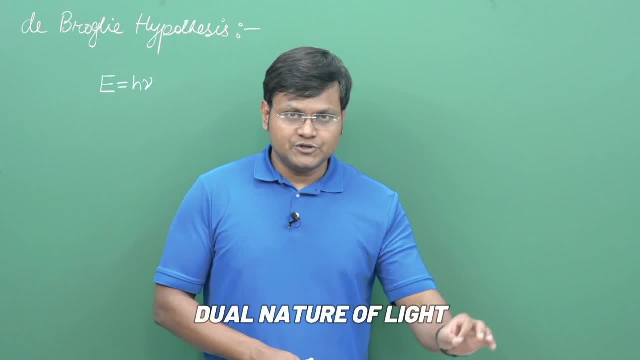 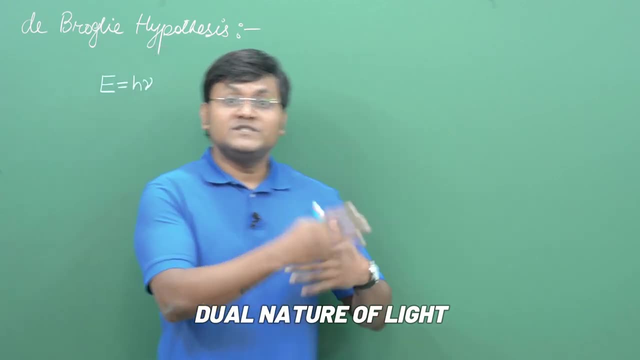 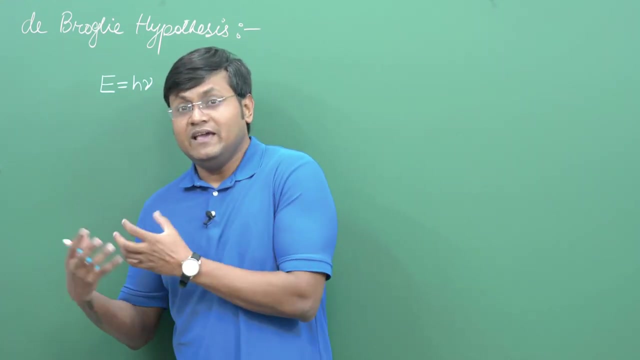 You see, this is not a mistake. This is not some exception. This is a general manner in which light behaves, That in certain circumstances it demonstrates wave properties, wave characteristics, and in certain circumstances it behaves like a particle. This is how light truly is, So 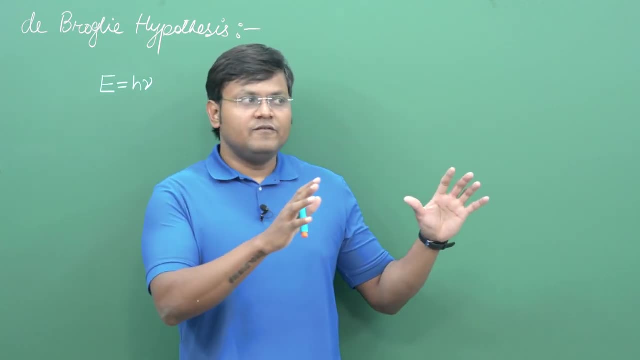 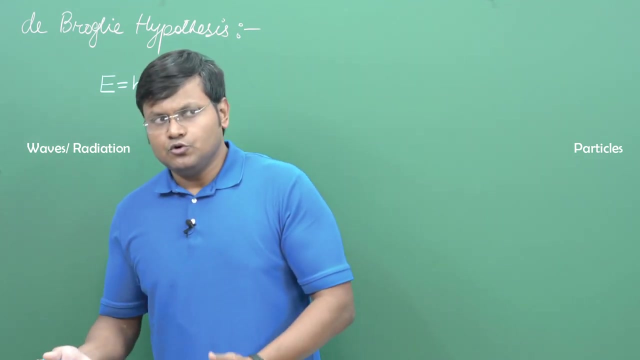 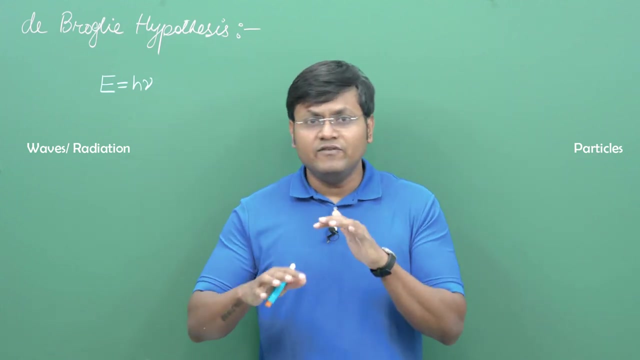 now the question is: the universe is composed of particles and radiation. Now, radiation has demonstrated dual nature, So do particles also have dual nature? Do traditional particles also behave in some wavy fashion? Well, the first time, the very first time this was proposed. 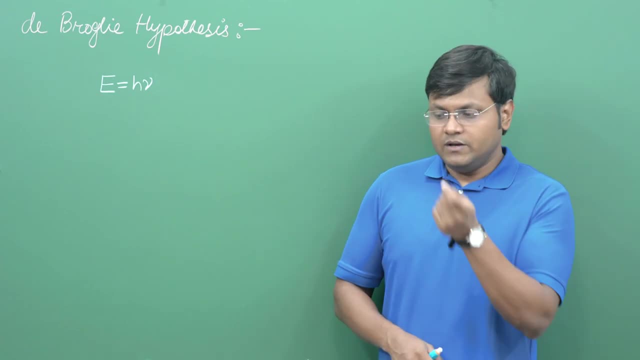 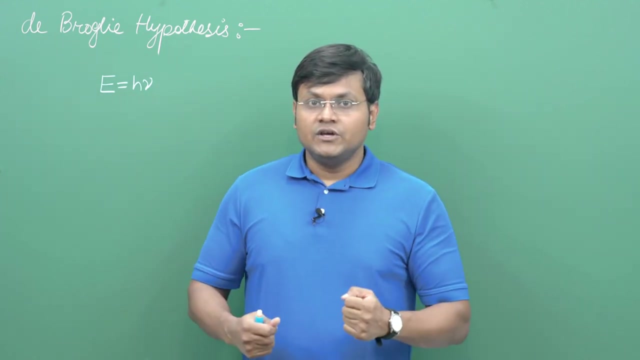 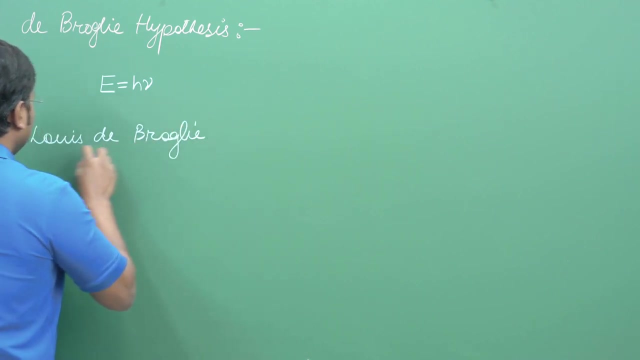 we did not have any kind of an experimental evidence to support it, But based on arguments of philosophy, arguments of a grand symmetry in our universe. It was proposed for the very first time by a physicist known as Louis de Broglie. Louis de Broglie, that is how we 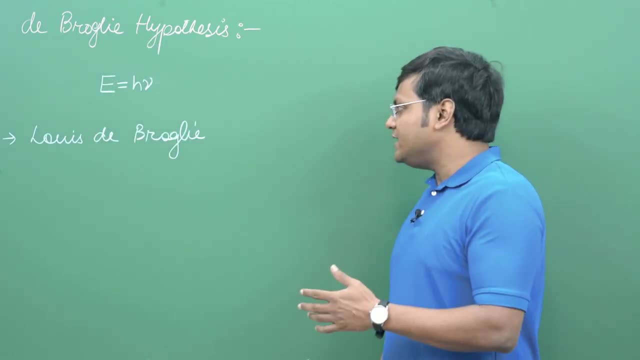 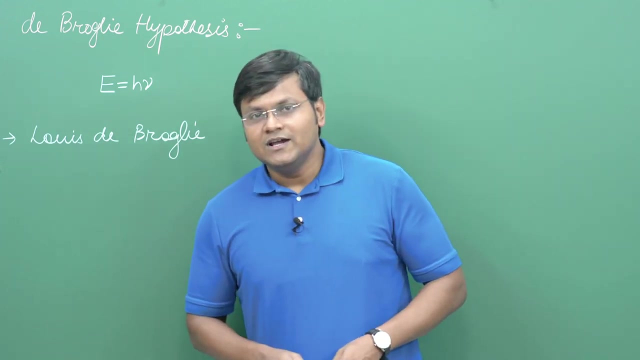 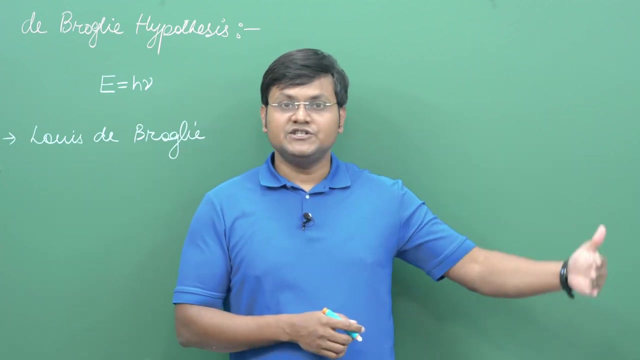 pronounce it, but he was a French scientist and the way to pronounce his name is Louis de Broglie. He was a history student who was very much attracted to these questions, these philosophical questions about physics and nature. at that point in time- And he in 1924,. 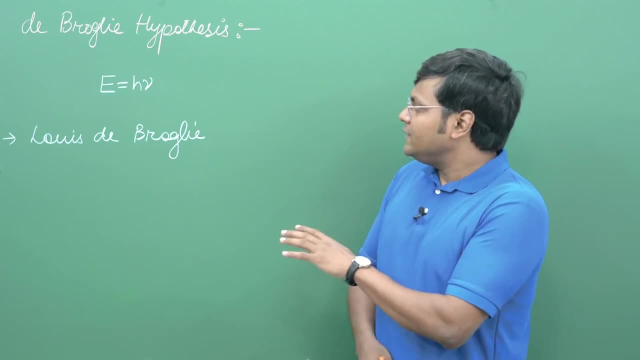 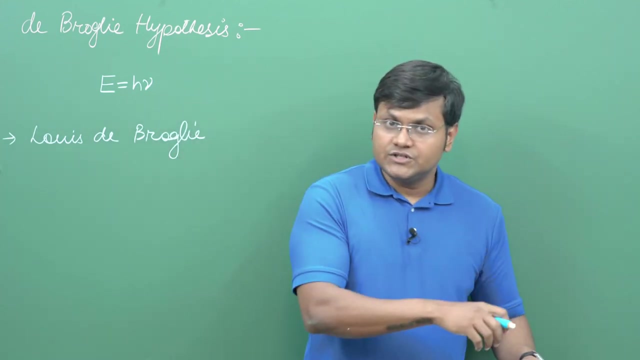 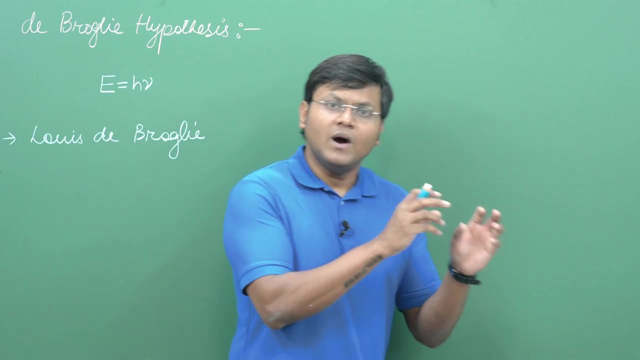 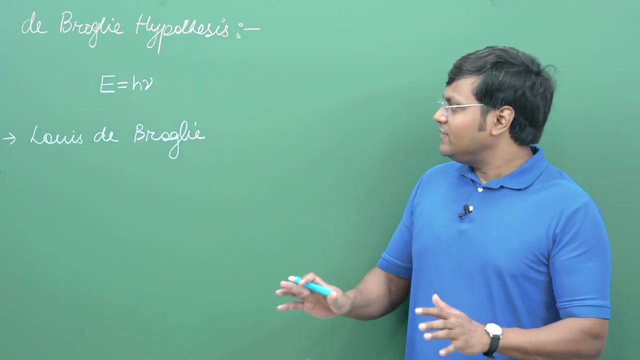 in his doctoral thesis proposed that just like photons or just like light, there is a dual nature. Particles, traditional particles, like electrons, also have a dual nature, That electrons also behave like particles in some circumstances and waves in other circumstances And we can figure out what is the wavelength of that kind of a particle or a matter wave. 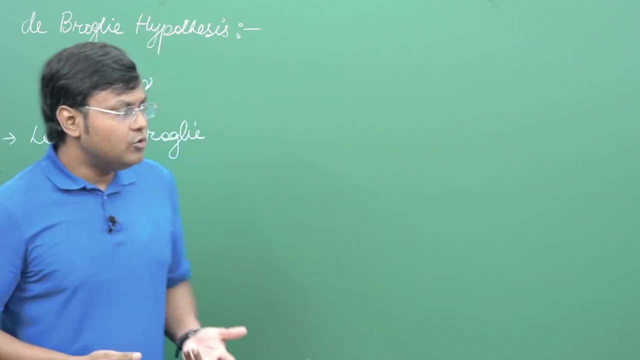 based on our understanding of the relationships of a photon. So, for example, the energy of a photon is given by E equals L, H, nu, And the momentum of a photon is given by E is equal to or P is equal to E upon C. 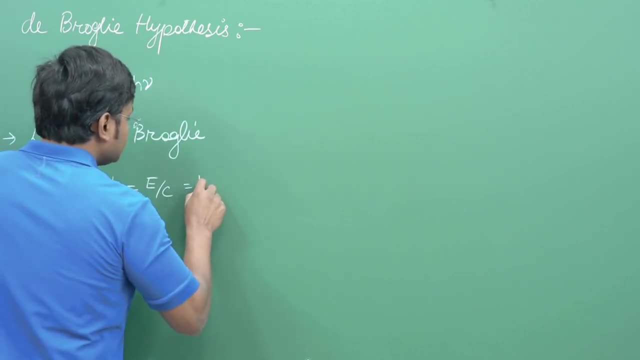 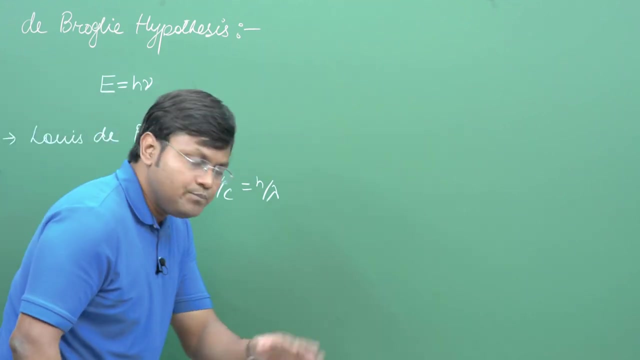 So if I substitute E is equal to H, nu. here this becomes H, nu upon C. But what is nu upon C? Nu upon C is 1 upon lambda, because C upon nu is lambda, So this comes out to be H upon lambda. So you see that, for a photon at least, the relationship between the momentum of a 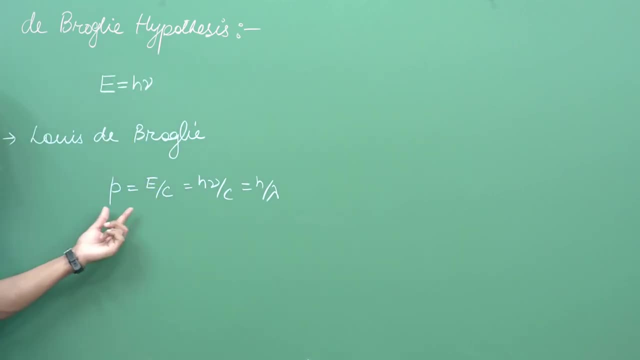 photon, and the wavelength is given by this, That the momentum of a photon is inversely correlated with the wavelength of a photon. What Louis de Broglie suggested was that even for particles. so the de Broglie hypothesis suggests that for particles like electrons, 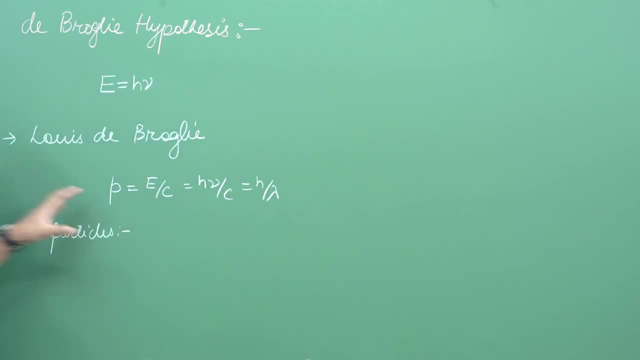 protons, neutrons, even atoms. this kind of a relationship holds true. That means even particles have a wave associated with its motion and the wavelength of that matter wave. Ok, So if I can call it as such, if I can say matter wave, if a particle has a wave. 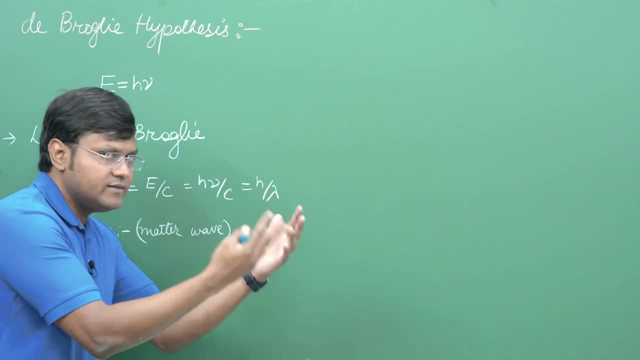 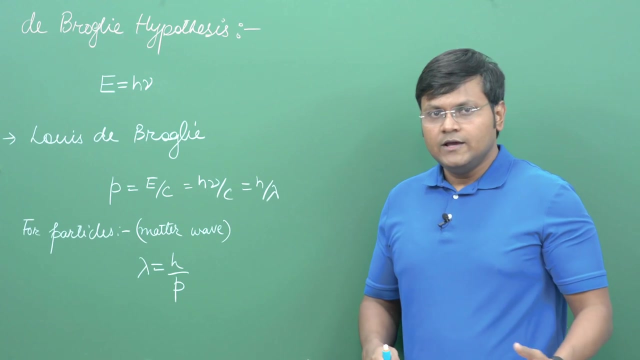 associated with it. Let me call it a matter wave. Then the wavelength of that matter wave is given by lambda is equal to H upon P- This is the de Broglie hypothesis- That, just like light, has a dual nature of its own. behaves like a wave, behaves like a particle, sometimes. 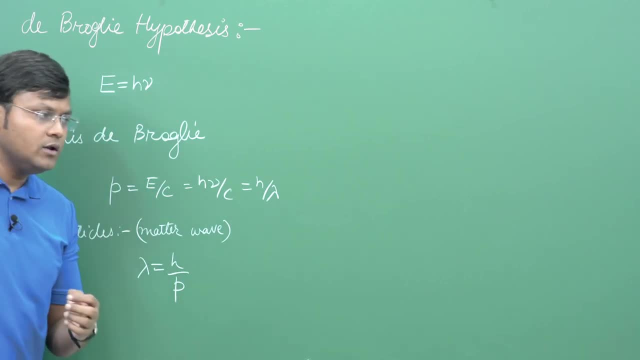 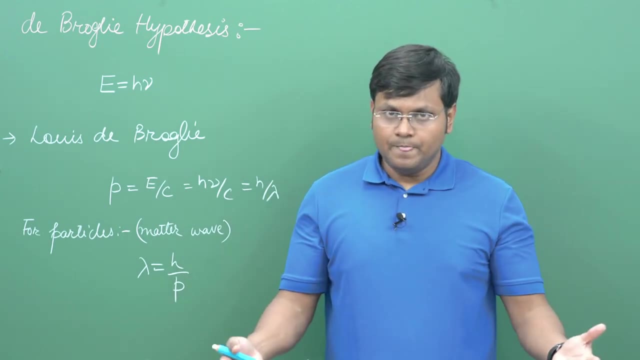 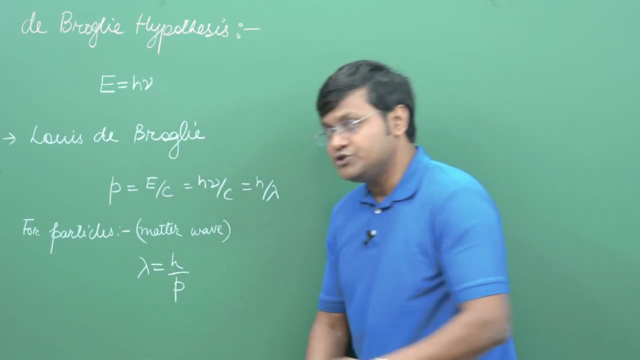 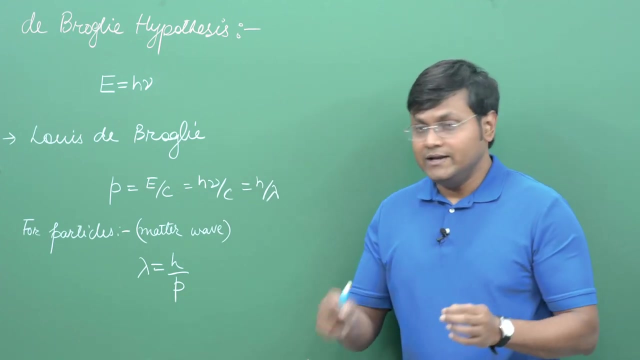 and these relationships hold true for light photon. in that same fashion even particles. a matter has this kind of a dual nature that it has a certain momentum associated with its motion and it also has a wavelength associated with the matter, wave associated with its motion, and the wavelength and the momentum are inversely correlated. so the wave property 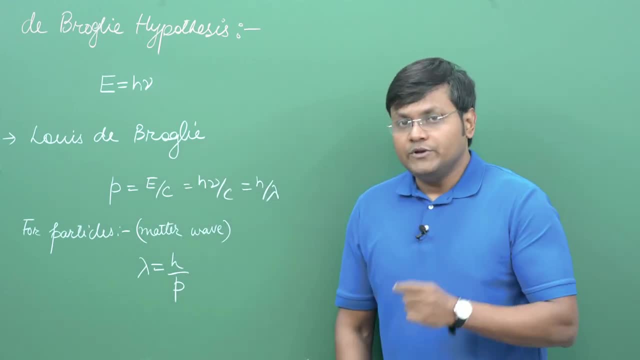 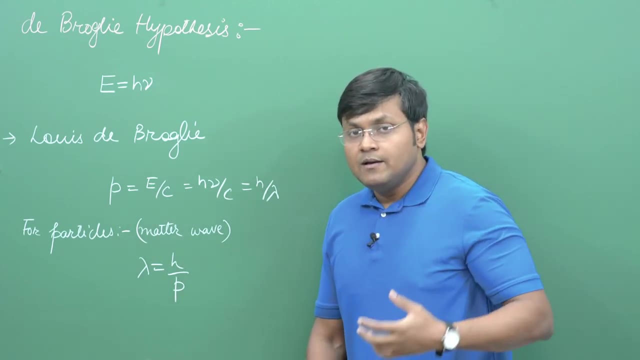 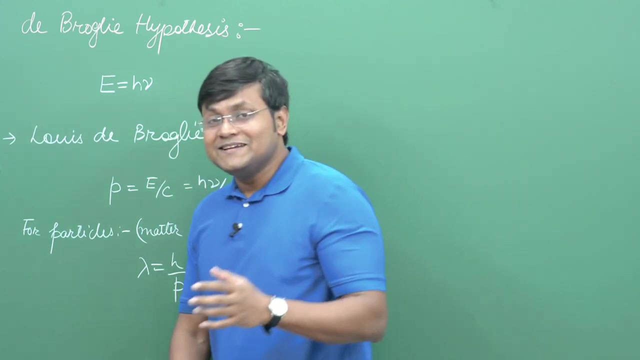 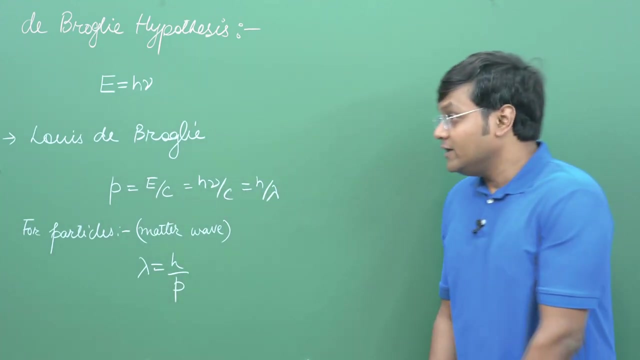 is inversely correlated with the particle property. so the duality of waves and particles that is demonstrated by radiation is not some exception, but in fact it is a general characteristic of particles and waves in this universe. since the universe is composed of particles and waves, both waves and particles demonstrate this kind of a dual behavior. that is what the 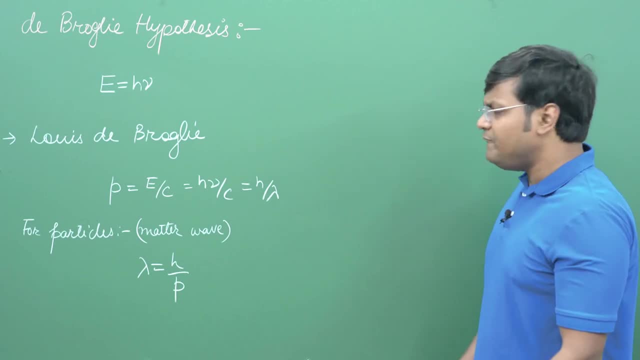 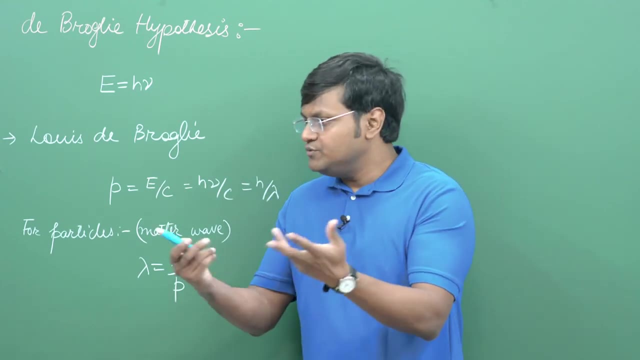 broad-spectrum wave is and the wave property is inversely correlated with the particle property, has suggested all right. now the question is, if particles do indeed have this kind of a wave nature, why don't we see that in our day-to-day life? i mean, i have these objects in my hands. 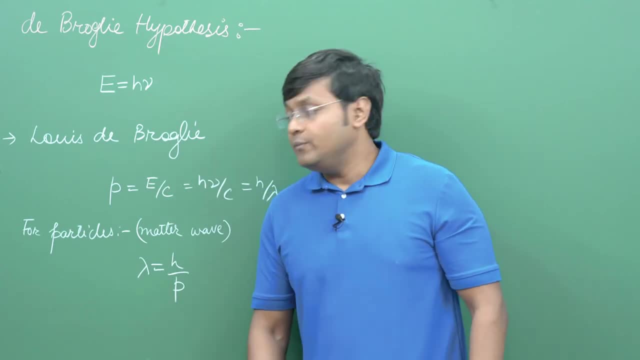 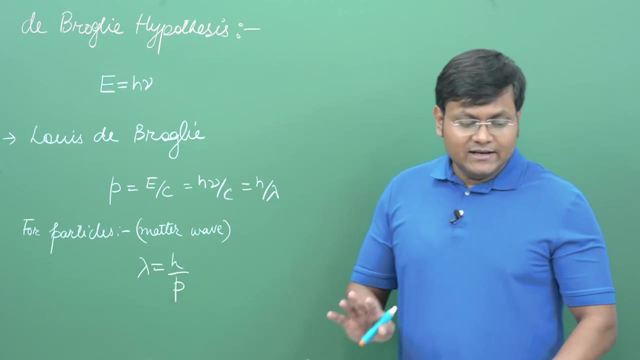 right, they are particles, right. why don't they demonstrate wave behavior? well, the answer to that question comes if we actually start making measurements. so let's look at this expression in a little bit more detailed fashion, all right, so the expression given by louis de broglie is: 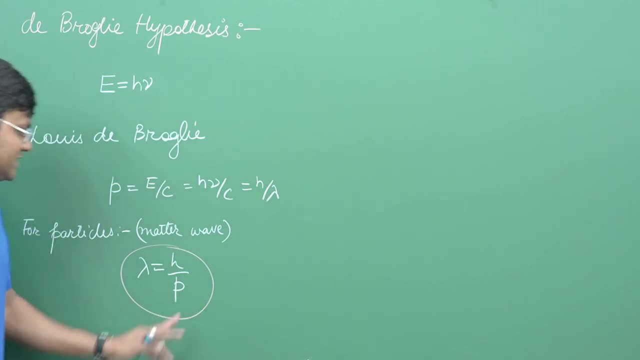 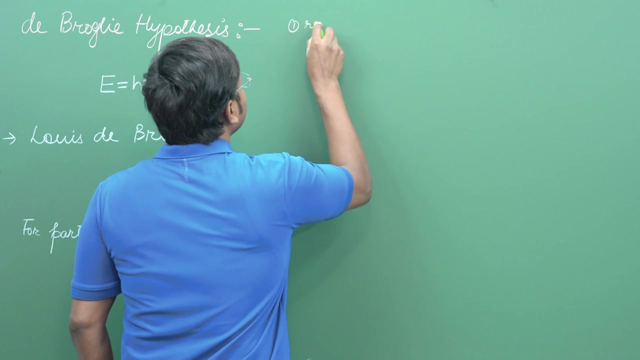 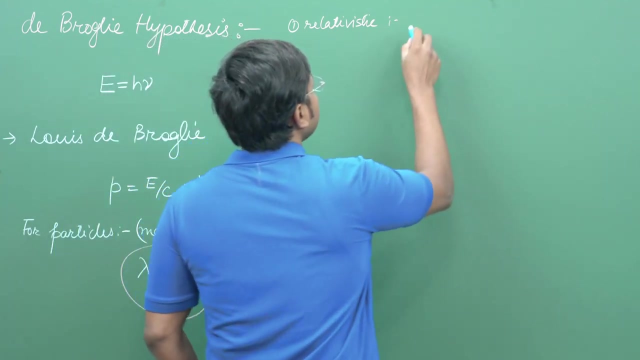 lambda is equal to h upon p. so what is p? p is momentum. if i write what momentum is for particles that are not traveling at very high speeds, it is simply m, v. but what if particles are traveling at very high speeds? so first let's look at relativistic case. in the case of relativistic scenario, the momentum actually 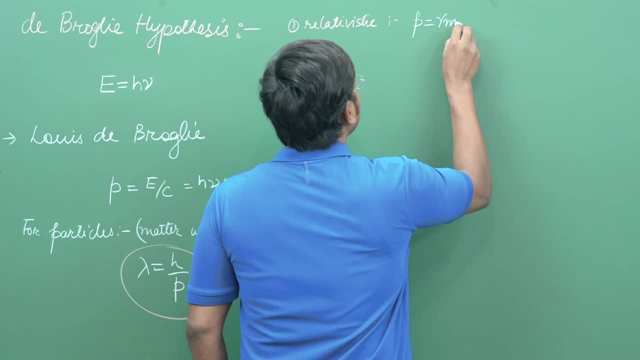 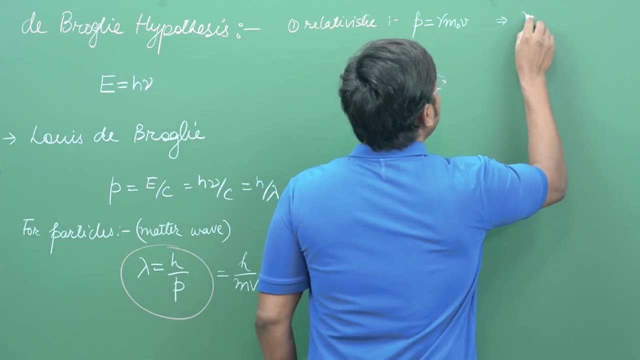 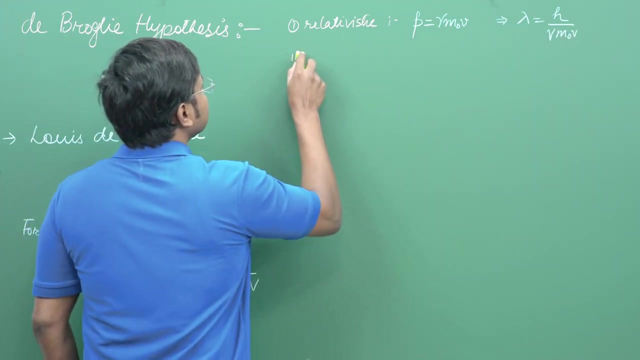 comes out to be what p is equal to gamma m, not v, where gamma is the gamma factor, 1 upon root over 1 minus v, square upon c square, and the momentum is equal to gamma m, not v, where gamma is the gamma and hence the lambda is actually equal to h upon gamma m, not v. and for non-relativistic cases, 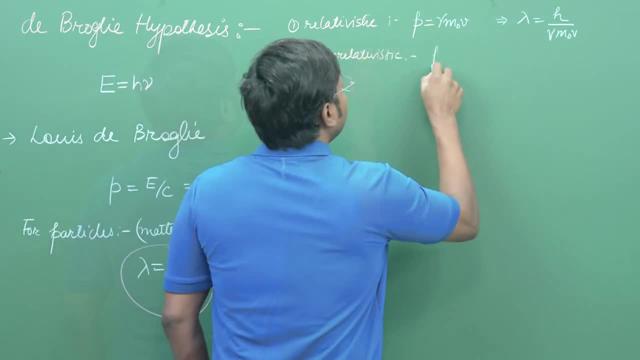 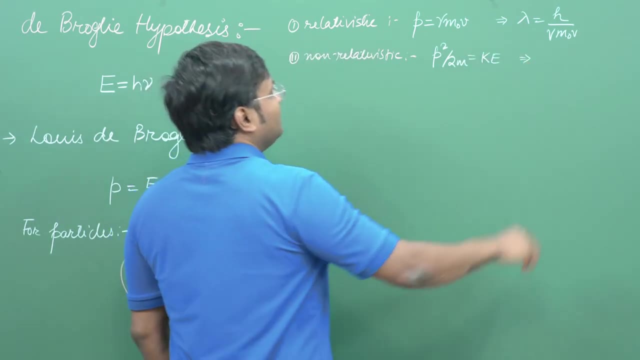 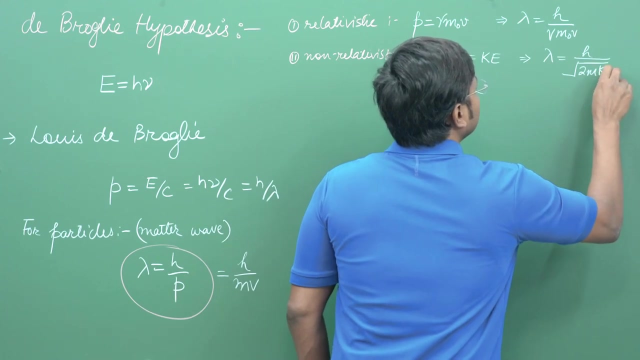 the momentum p square upon 2m is equal to the kinetic energy. right? so we can write the de broglie wavelength as lambda is equal to h upon root over 2m kinetic energy. so this is the original equation, but you can represent this as the original equation. so let's look at the. 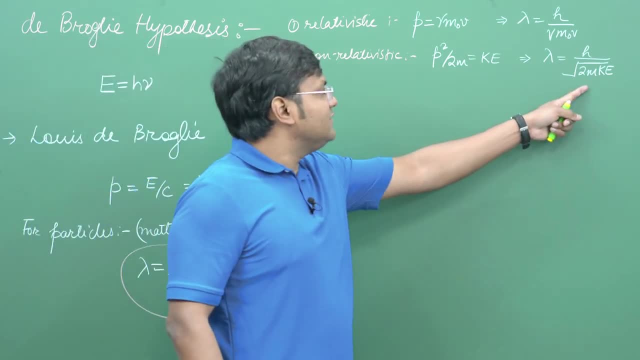 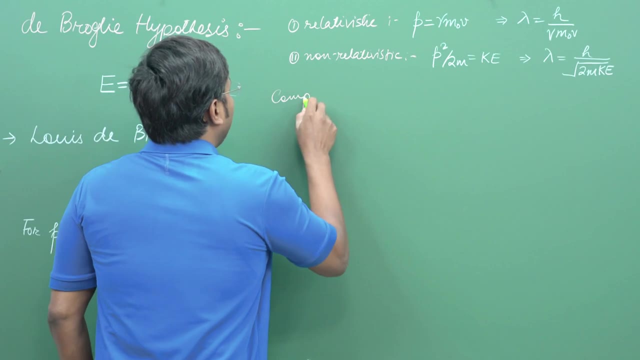 whatsapp score. here, as we can see, the velocity is basically the same as the velocity of the energy drop, and which is equal to the velocity of the energy drop as well. the velocity of the energy drop is the same on this particular situations. as you can see, on this particular 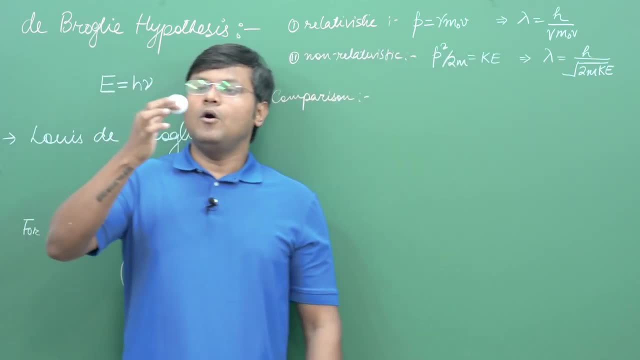 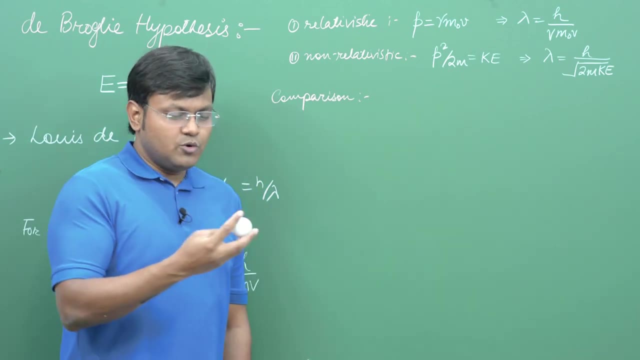 situation. the velocity of the energy drop is very different, as we can see in this specific situation. so what is p? p is welcome. this is what we are getting from all the. this is what we want to know. so the value of p? p, as we are attacking now, is equal to m of g by h upon. 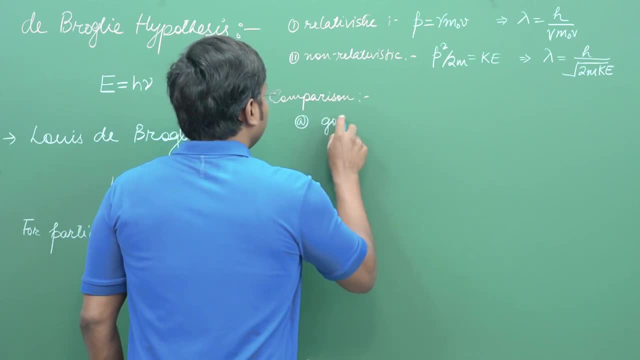 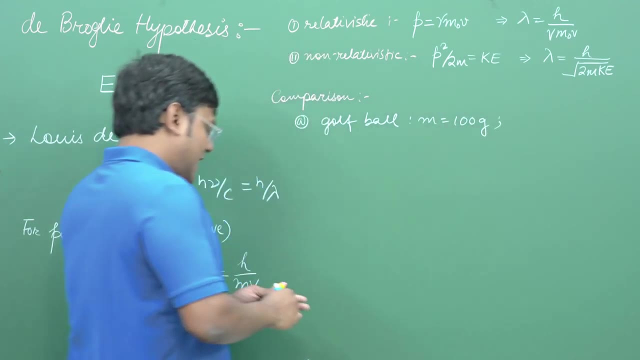 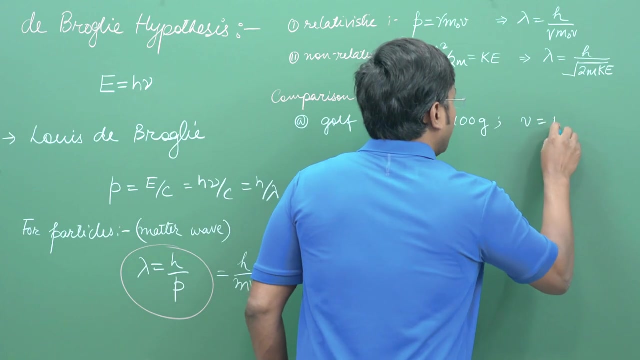 So let's say I have a golf ball, okay, whose mass is 100 grams, and maybe I throw it. all right, I throw it at some speed of, let's suppose, 100 meters per second. then what is going to be the de Broglie wavelength associated with the matter, wave corresponding to the 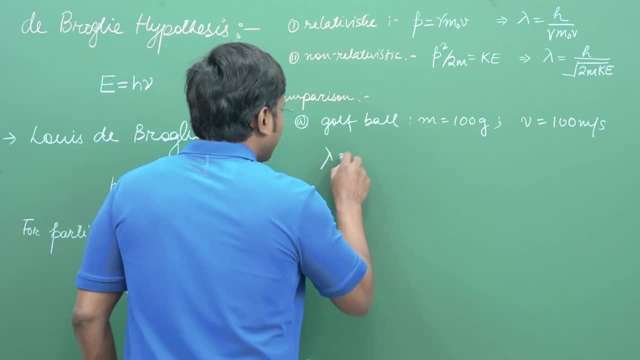 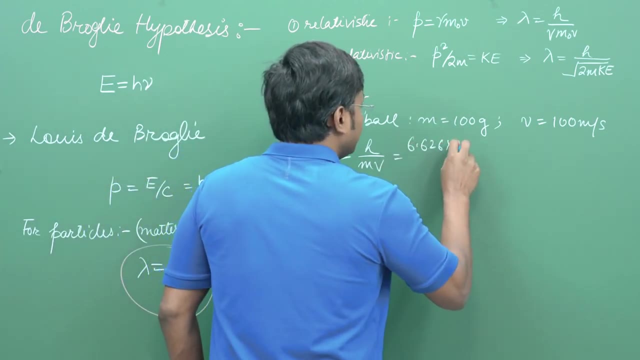 motion of this golf ball through air. So if I calculate that it comes out to be what is h, h is a Planck constant 6.626 into 10 to the power minus 34 joule. second, divided by mass is 100, so 100 times 10 to the power minus 3 into velocity, is 100. 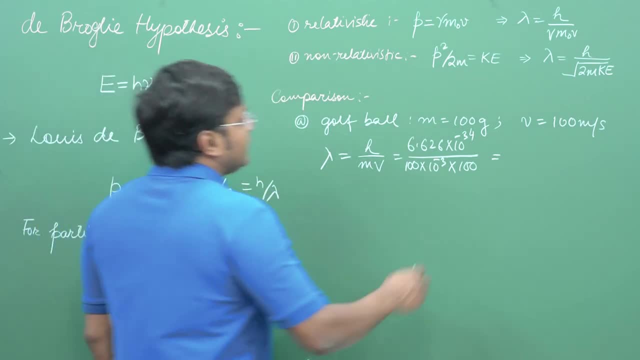 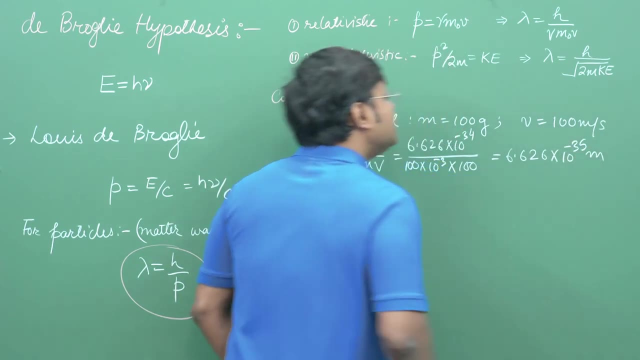 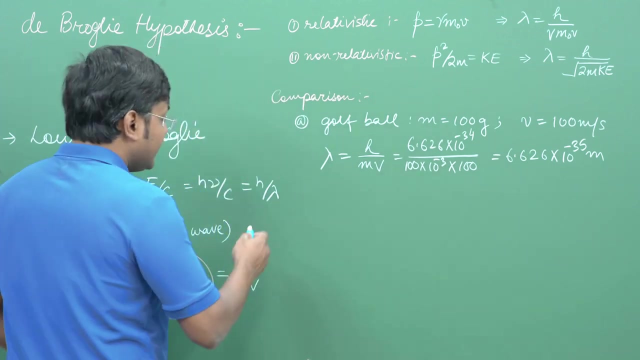 So this comes out to be around 6.626 into 10 to the power, minus 35 meters 6.626,. I'll just keep that here. let me do another calculation first. The second is electron. so let's suppose I have an electron, I don't have an electron. 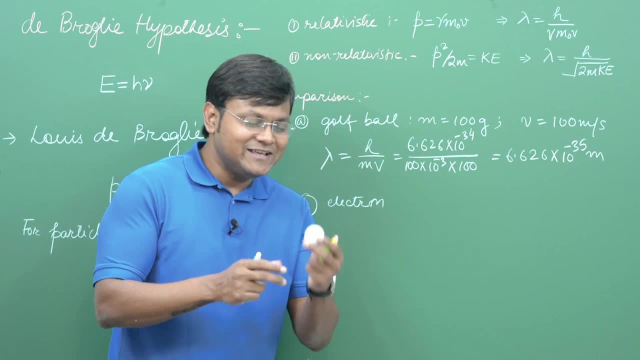 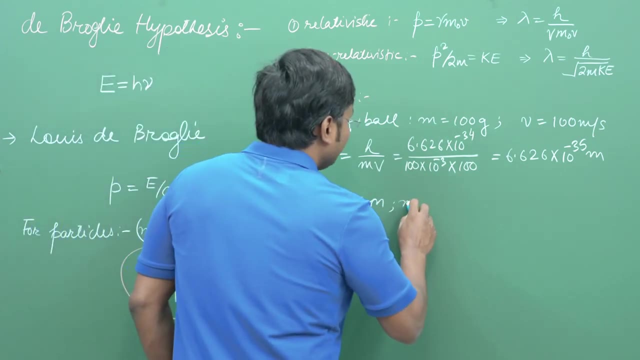 in my hand. I mean, I do have electrons in my hand, but I'm not carrying it like this ball because it's too small to carry. okay, So, electron, it has a mass of around 9.1 into 10 to the power, minus 31 kgs. and let's 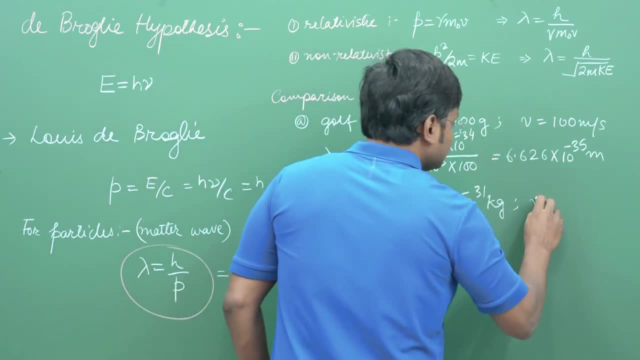 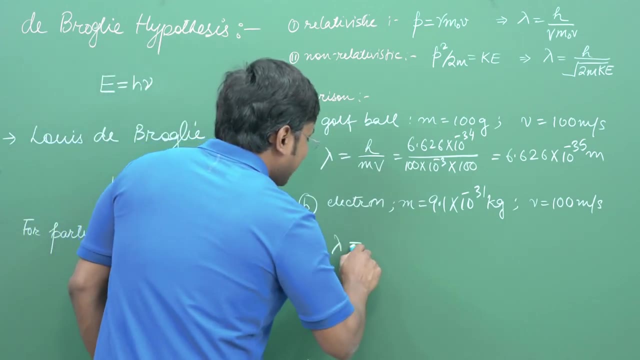 suppose electron is also traveling with a second, It's the same velocity. okay, v equals, so it's a non-relativistic scenario. 100 meters per second is very low compared to the speed of light, So what is the lambda in that situation? 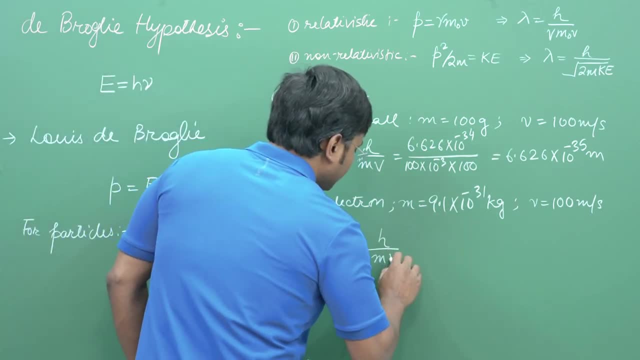 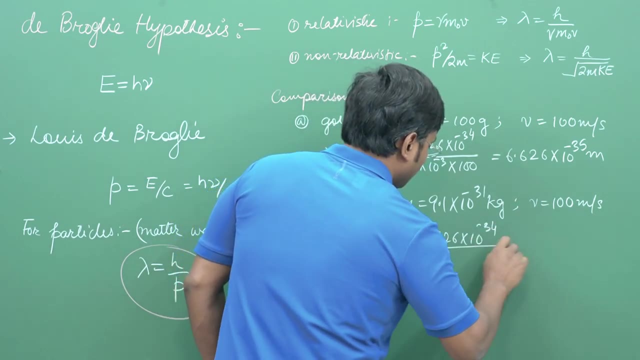 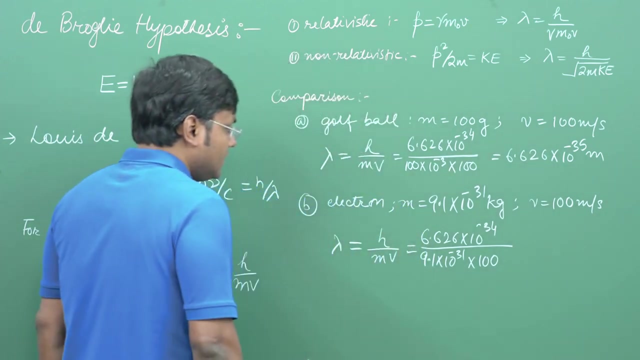 The lambda in that situation comes out to be h upon mv. so if I again rewrite these values divided by 9.1 into 10, to the power minus 31, multiplied by 100 meters per second, so this comes out to be: I think I have. 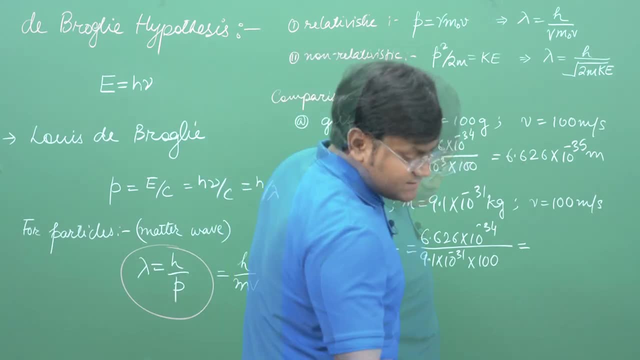 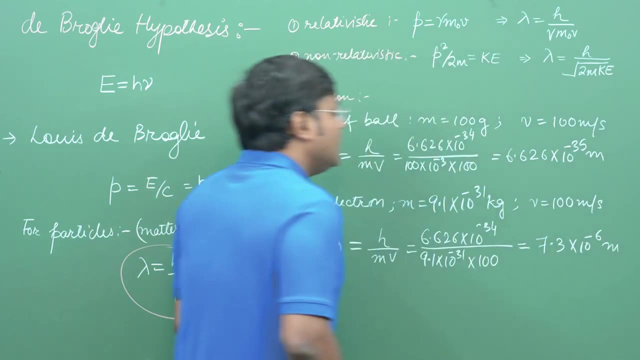 I have already done my calculation somewhere here. this comes out to be somewhere around 7.3 into 10 to the power minus 6 meters. Now two particles: a golf ball and an electron, both traveling at the velocity of 100 meters. 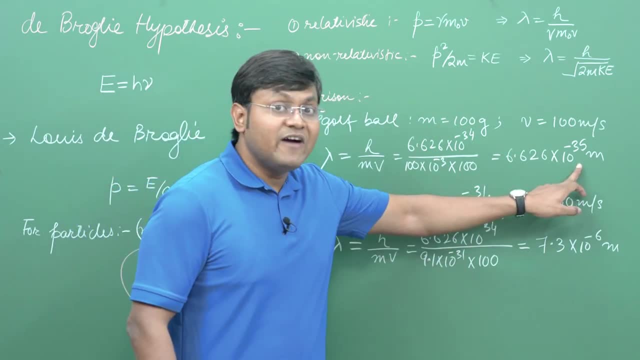 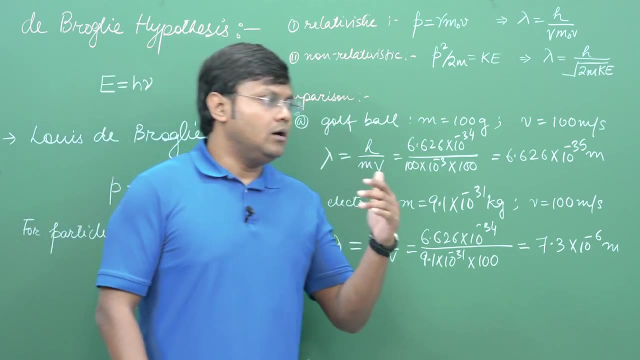 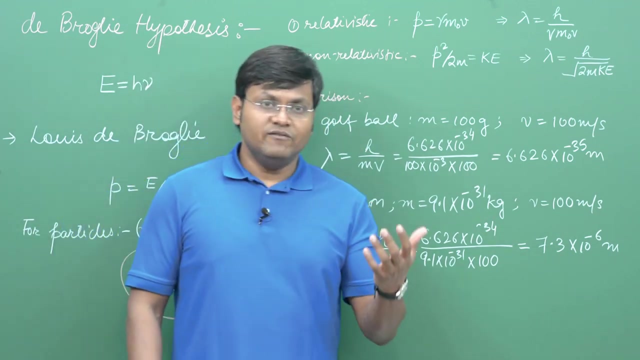 per second. one has a de Broglie wavelength of 10 to the power minus 35 meters. the other has a de Broglie wavelength of a few micrometers. You see, whenever we want to calculate the wavelength Of anything, any wave, then we need some instrument, some device that has an aperture. 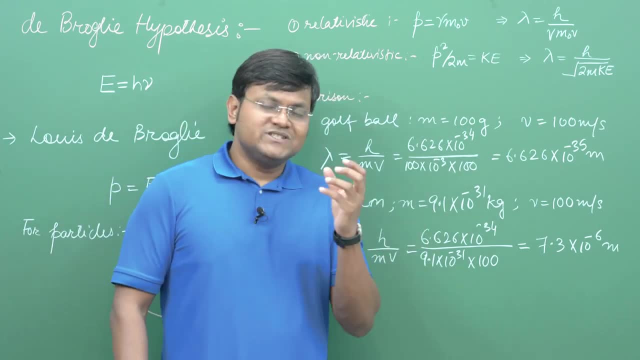 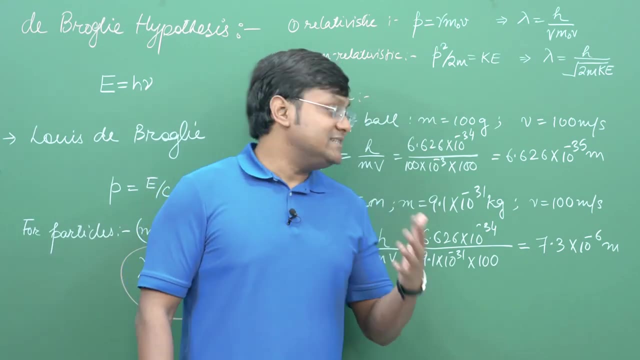 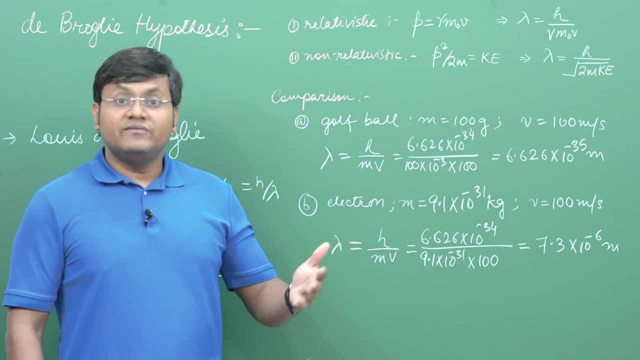 or some sort of a opening or an obstacle whose size is of the same order as that of the wavelength. Now, usually we are very capable of detecting wavelengths of this particular order. You see, even light, visible light, has a wavelength of around 4,000, 5,000, 6,000 angstroms right. 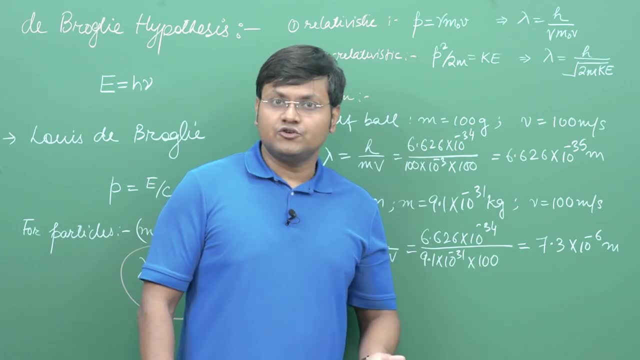 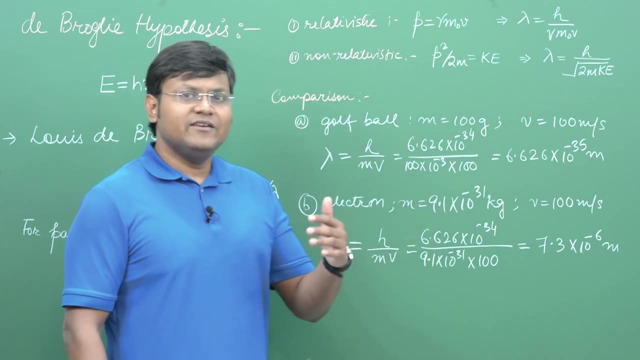 If you look at x-rays, they have wavelength of a few hundred angstroms. Okay, If you look at gamma radiation, maybe a few angstroms or even less than that. right, So we are capable of detecting radiation which has wavelength of this particular order. 10. 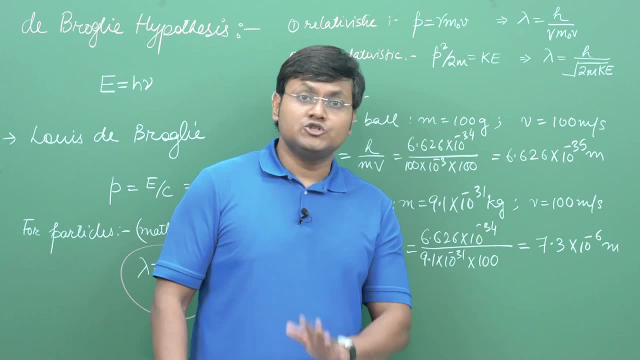 to the power minus 6,, up to maybe 10 to the power minus 11, even 10 to the power minus 12 meters. right, But if you make this comparison with this number, 10 to the power minus 35, that is. 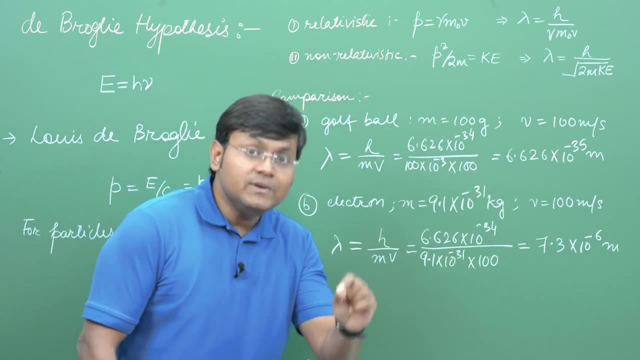 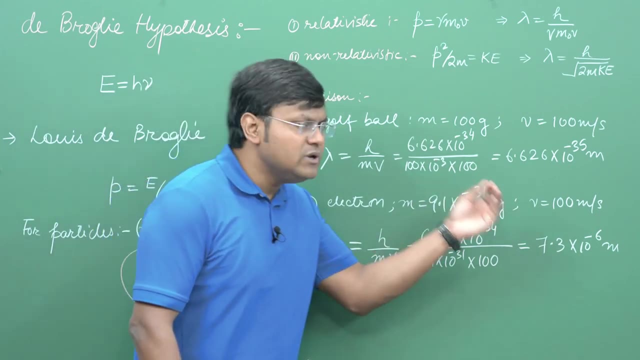 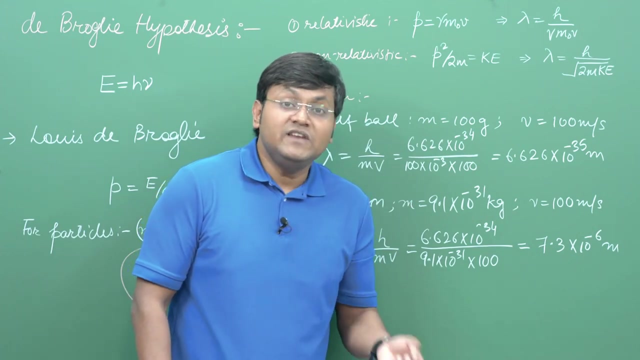 extremely small, That is extremely, extremely tiny. It is in fact so tiny that there is no instrument or device that can actually measure the wavelength. I mean, if you look at an atom, even the nucleus of this is of the size of around 10 to the power minus 15 meters: 10 to the power minus 15 meters. 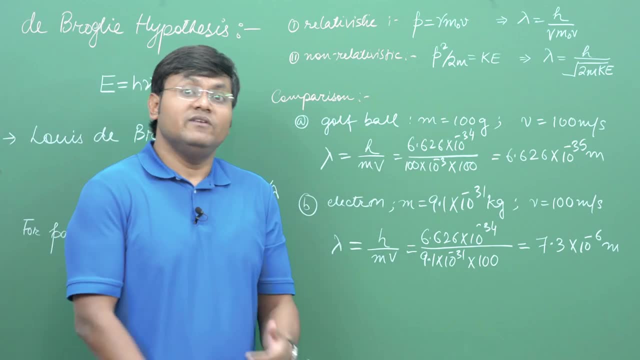 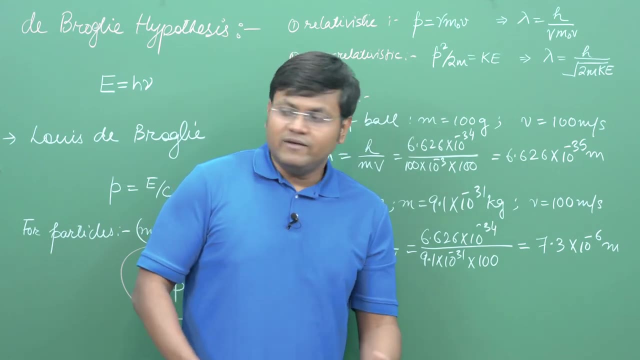 So this wavelength is many orders of magnitude smaller than even a nucleus. We don't have any instrument or a device to actually measure this kind of a wavelength, So therefore, whenever we deal with macroscopic particles, we don't really see the wave characteristic. 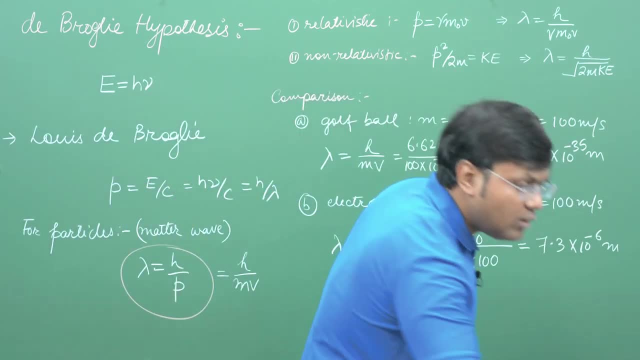 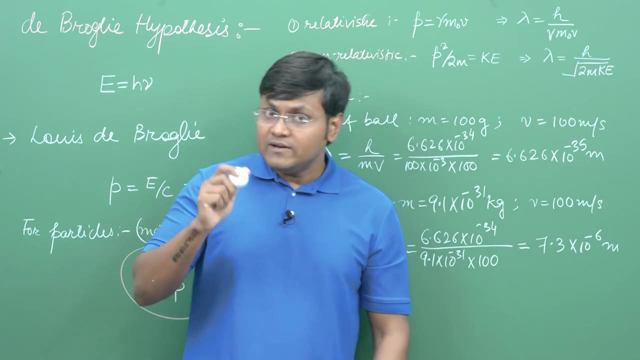 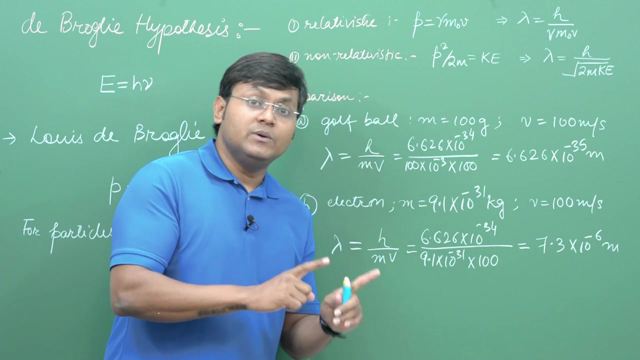 of those macroscopic particles. Okay, If I throw a ball, I don't really see any kind of interference phenomena or diffraction phenomena associated with the motion of this ball, because the wavelength associated with this is so tiny that it is almost negligible. However, when we do go into the microscopic domain where we encounter electrons, protons, 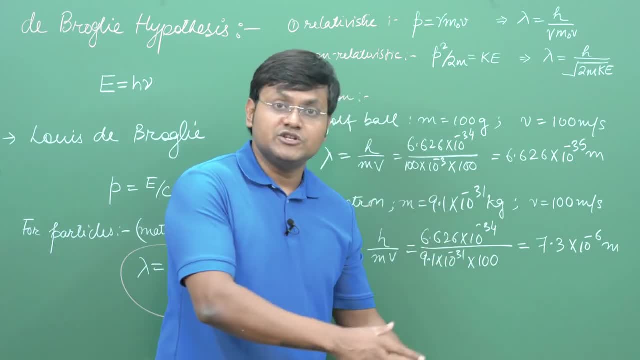 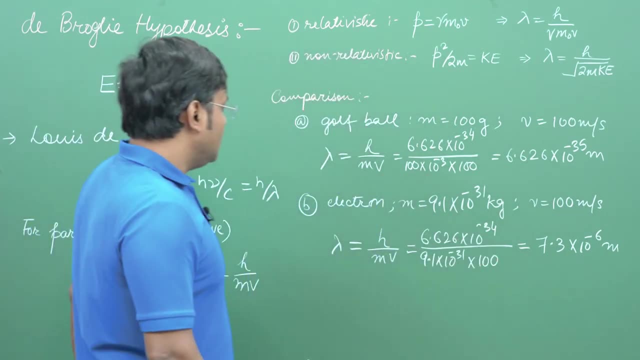 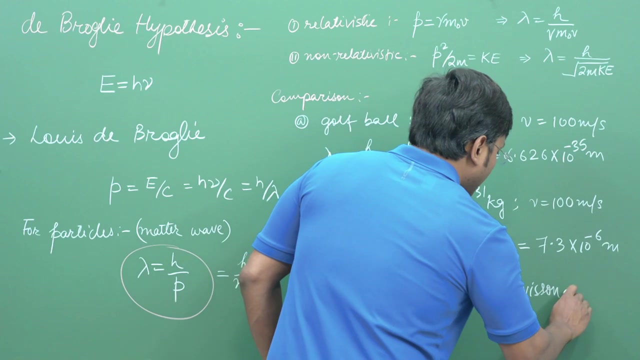 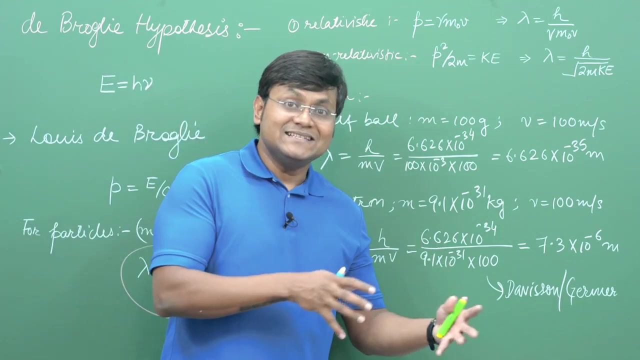 neutrons, even atoms. they in certain situations do demonstrate wave behavior, wave characteristics that can be detected. For example, we will study, We will study in the future lectures an experiment called Deveson and Germer experiment where when you bombard an electron beam onto a crystal lattice you see certain kinds of diffraction. 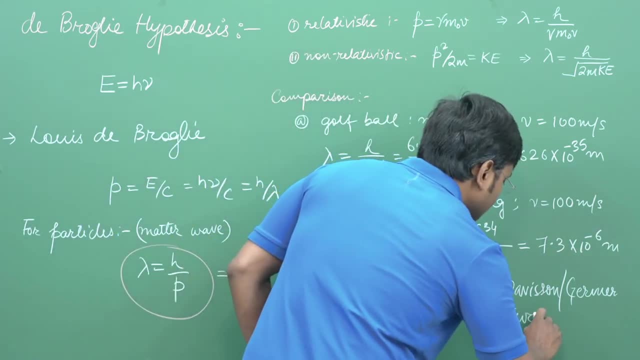 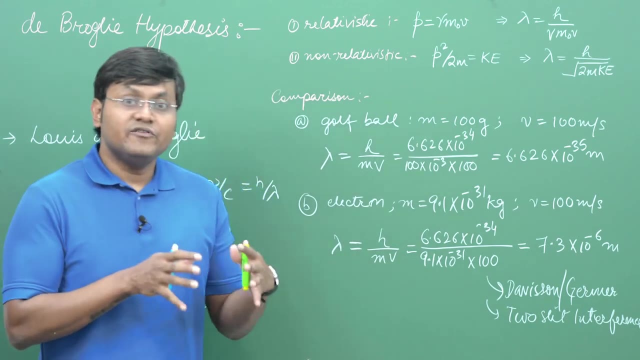 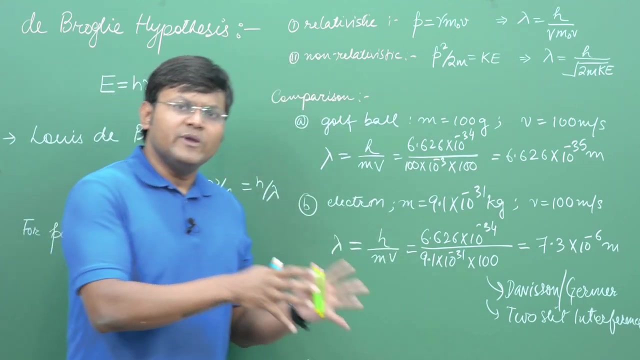 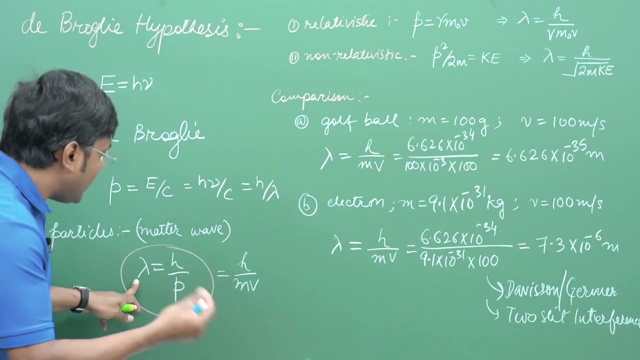 We will also see the two-slit interference experiment, where electrons demonstrate interference in the same manner that light demonstrates interference. Okay, So when we go into the subatomic particle, then the momentum becomes so small that the wavelength becomes sufficiently large that it is detected by instruments. 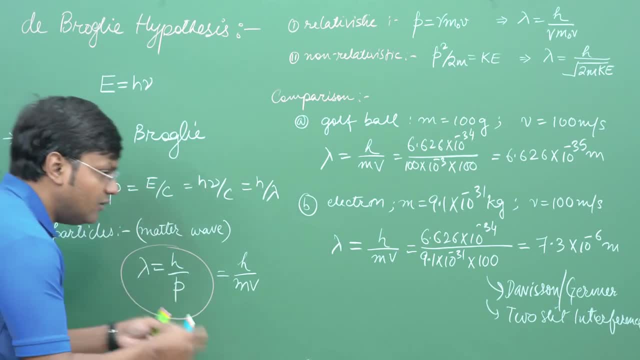 So you see this property. This property gives us an inverse correlation between the wave nature and the particle nature, Momentum being the particle nature, wavelength being the wave nature. So, when we go into the macroscopic world, the momentum becomes so high that the wave 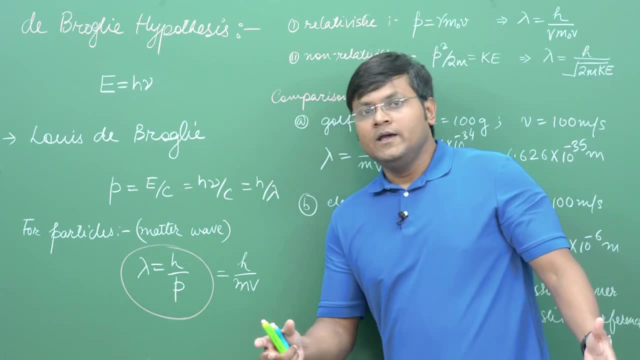 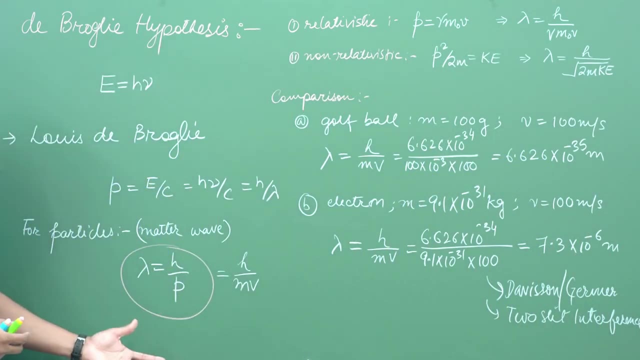 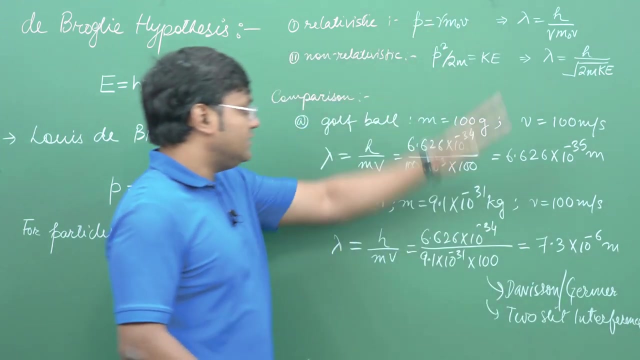 nature is almost negligible, We don't really see it. But when we go into the microscopic domain, then the momentum becomes less and we actually do end up seeing wave characteristics, which is interesting, because not only light demonstrates dual nature. even electrons demonstrate dual nature of particles and waves, which is going. 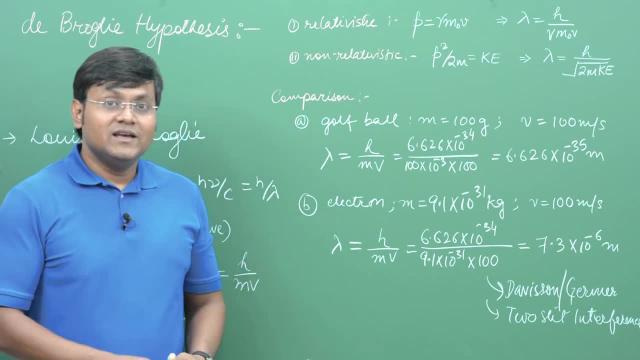 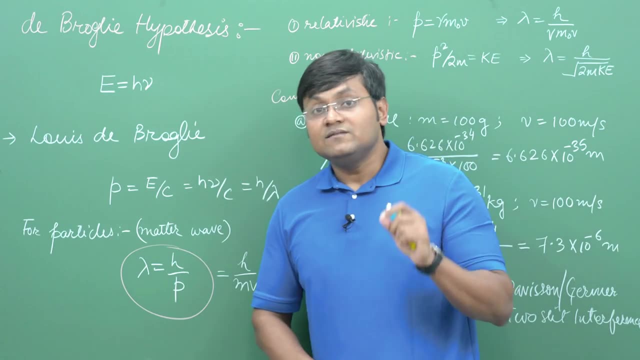 to be our starting point of quantum mechanics, Because, you see, one of the fundamental equations in quantum mechanics is the Schrodinger's equation and Schrodinger himself said that the fundamental equation of quantum mechanics is the Schrodinger's equation. And Schrodinger himself said that when he was formulating the Schrodinger's equation. 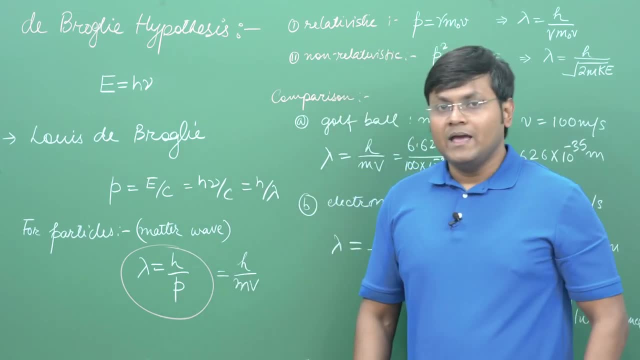 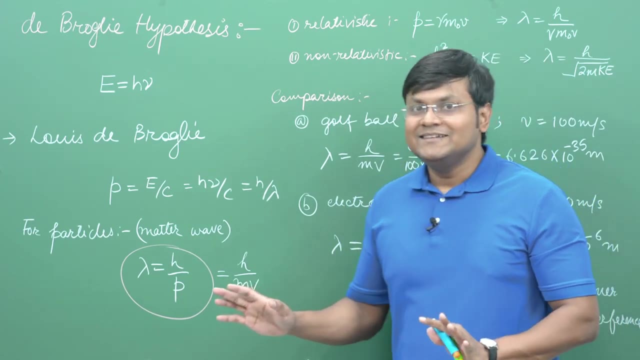 he took inspiration from the de Broglie hypothesis. I will not go so much into the detail right now. I will go in detail in the future videos. But yeah, the fundamental pillar of quantum mechanics, the Schrodinger's equation was: 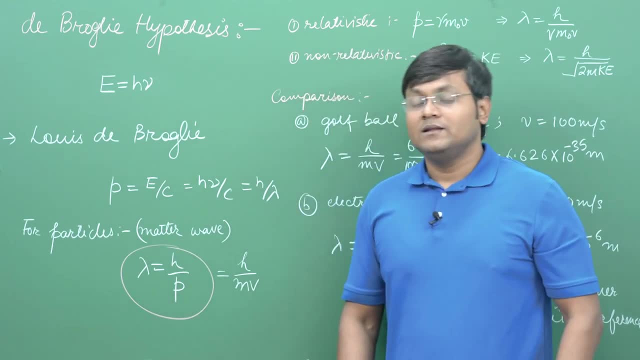 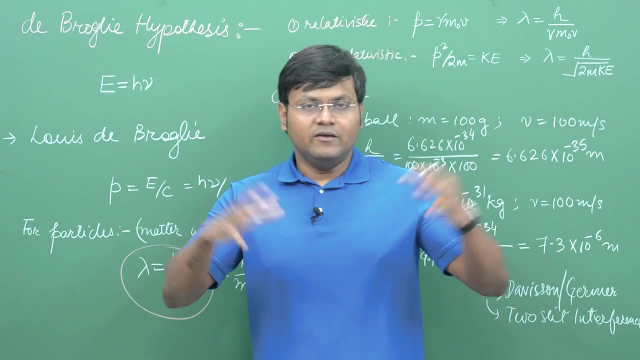 derived out of an inspiration from the de Broglie hypothesis. Now, the question may be: where did de Broglie get his motivation? Well, one of the answers, of course, as I said, these grand symmetry. We are in our universe of matters and waves having this kind of a dual nature. 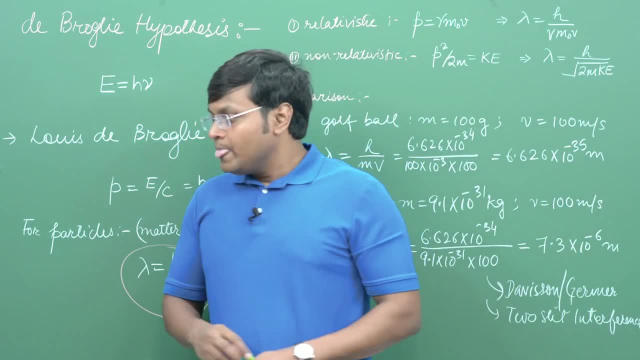 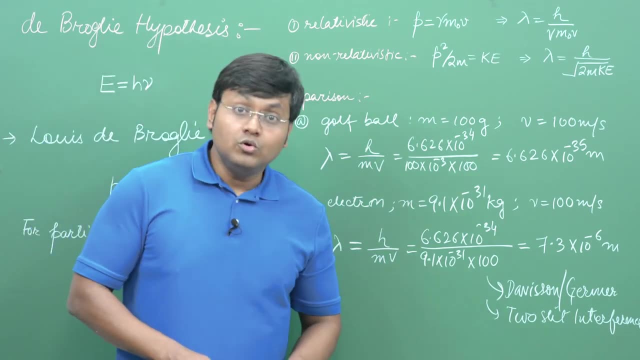 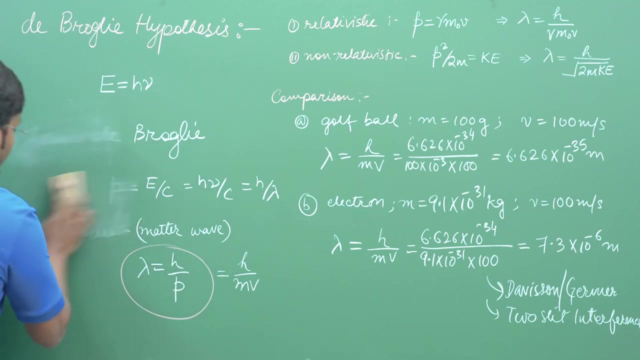 Also, if I may add one last point before I finish, this video de Broglie was also heavily influenced or inspired by what is known as the Bohr's condition of stability in atoms. When Niels Bohr gave his explanation for the OHm-G Winter Sensor and the Bohr's condition. 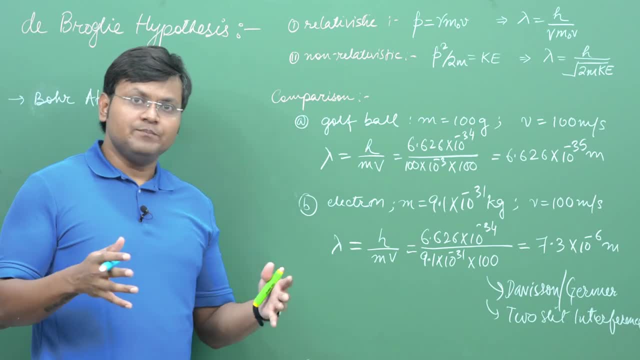 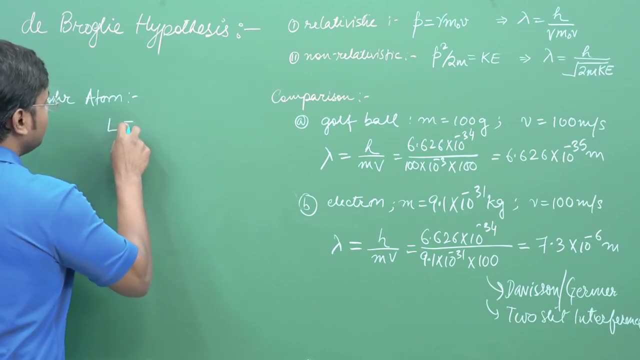 of stability in atoms. for the orbital stability of an atom he gave one rule. i won't go too much into the detail in the rule, i'll just mention it. he said that the angular momentum of an electron which is revolving around the nucleus in an atom is actually equal to integral multiple of h upon 2 pi. he gave this. 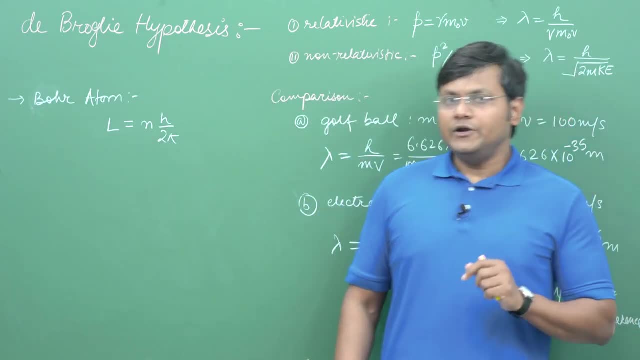 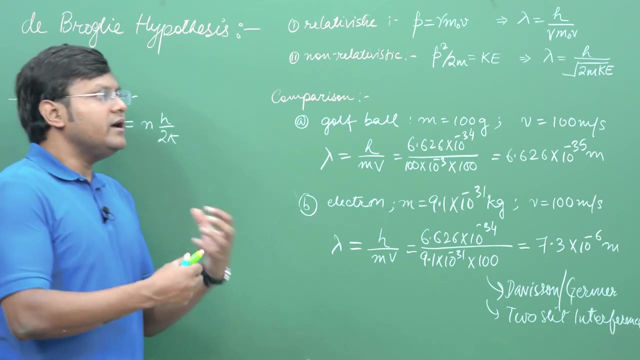 particular rule, and de broglie was quite inspired by this particular rule, because you see that what de broglie suggested was that there is a certain occurrence of these kinds of periodicities whenever we are dealing with matter particles. you see, periodicity is something that arises. 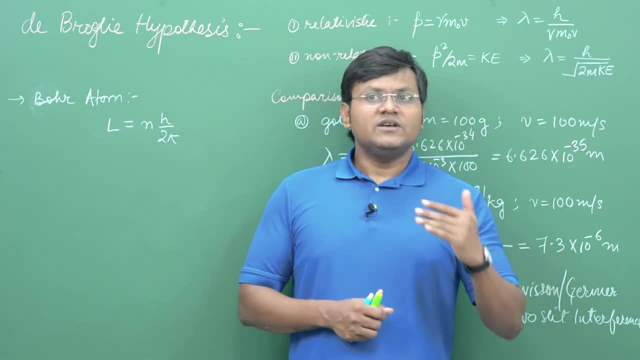 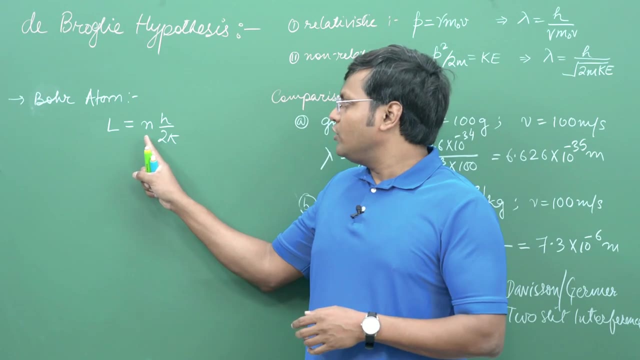 whenever we deal with waves, naturally, but it doesn't necessarily arise when we deal with particles. but in the atomic world these kinds of periodicities- by periodicity i mean the n, here the integer, integral multiple of quantities- these things are arising when we are trying to explain. 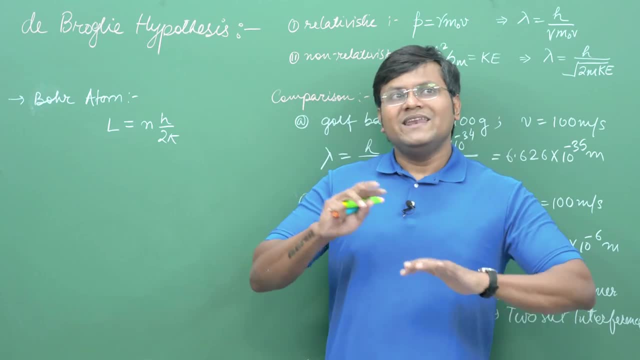 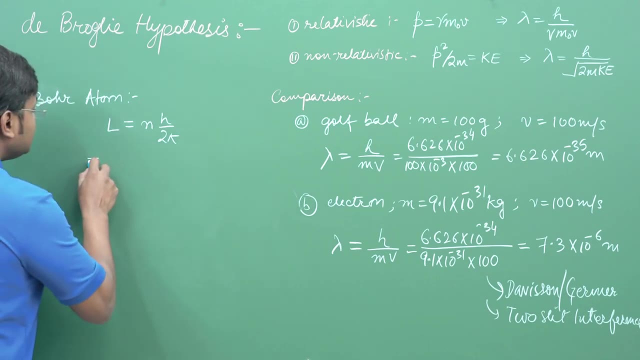 the behavior of particles. so that means the particles are somehow you connected with the motion of a wave. and i can explain that if we assume that the de broglie hypothesis is true. why? because the angular momentum of an electron around the nucleus is given by m v r, mass of the electron, velocity of the electron around the nucleus in its orbit. 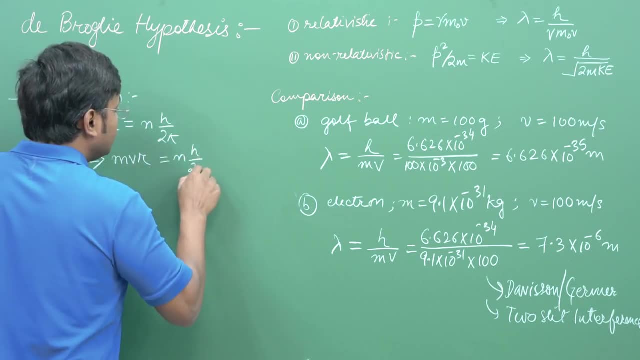 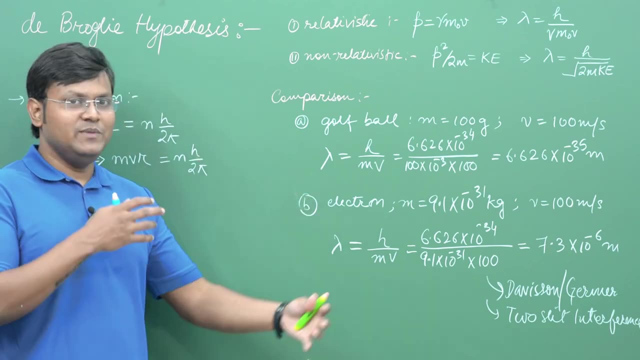 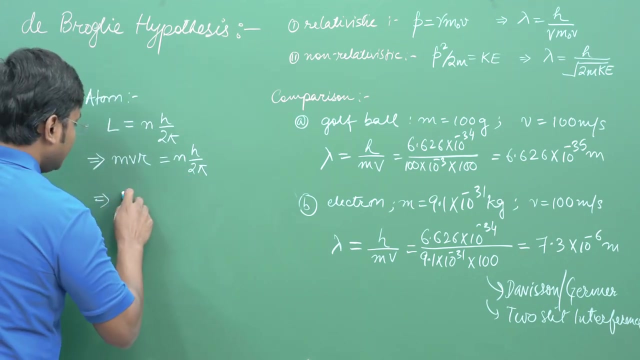 radius of the orbit is equal to n h upon 2 pi. if i just rearrange the terms a little bit, we will see why the bohr postulate become famous, and we will also see why de broglie hypothesis makes sense. you see, if i take 2 pi r to this side, i end up getting 2 pi r is equal to: 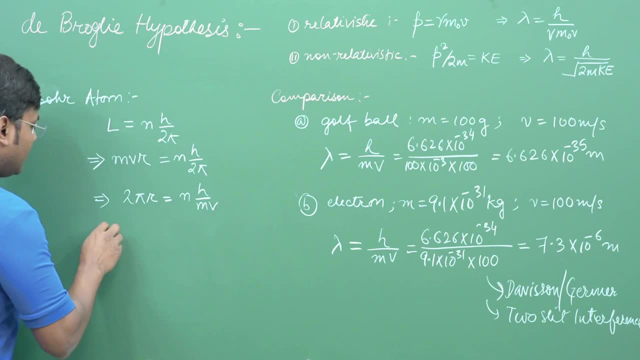 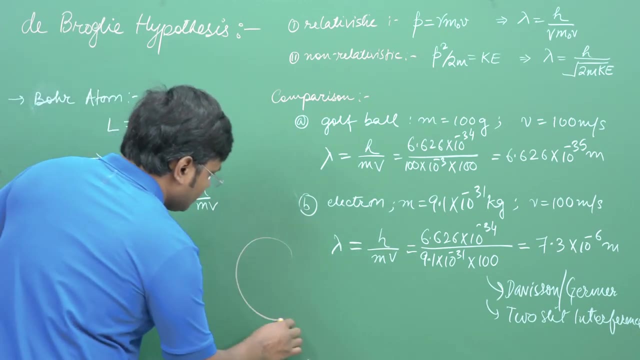 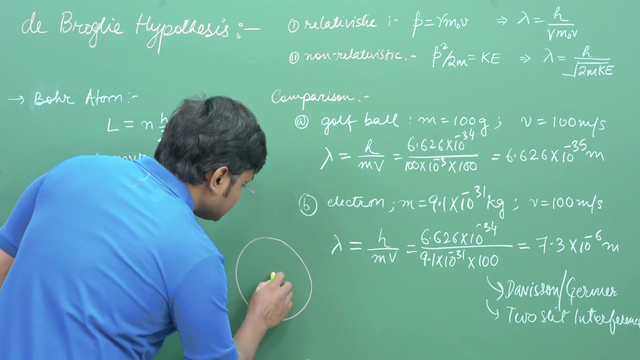 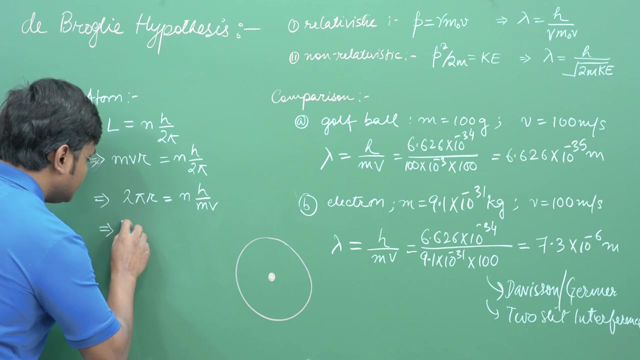 n upon h upon mv. what is 2 pi r? if you look at an atom, all right, let's suppose that i have this atom, okay, and this circle is the orbit of an electron around the nucleus. let's suppose this is the nucleus. in that situation, 2 pi r represents the circumference, right circumference of the orbit. what is h upon mv? 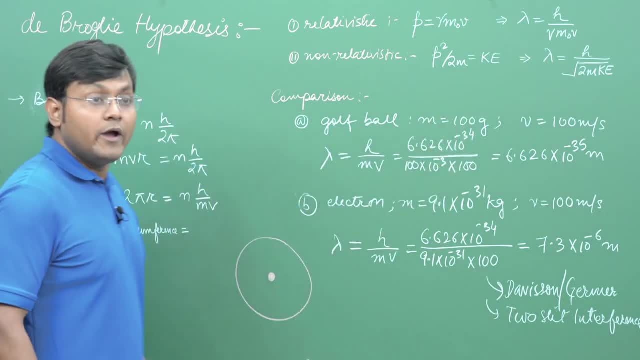 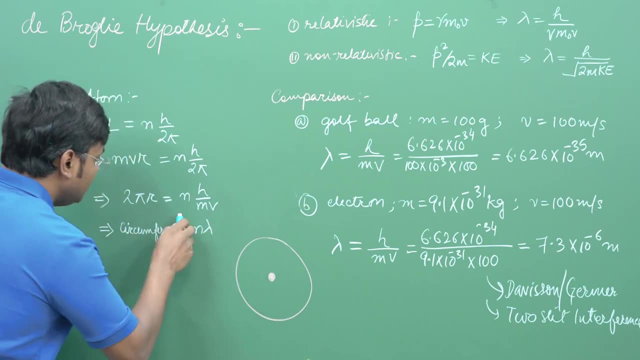 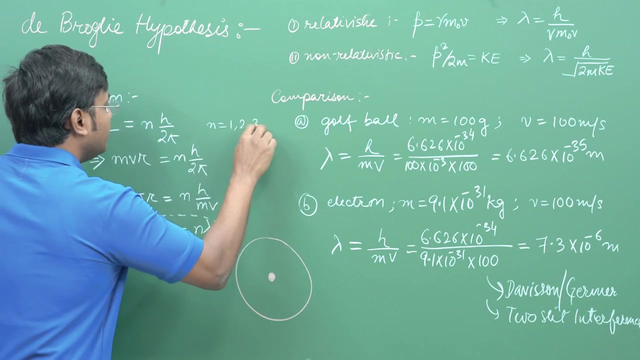 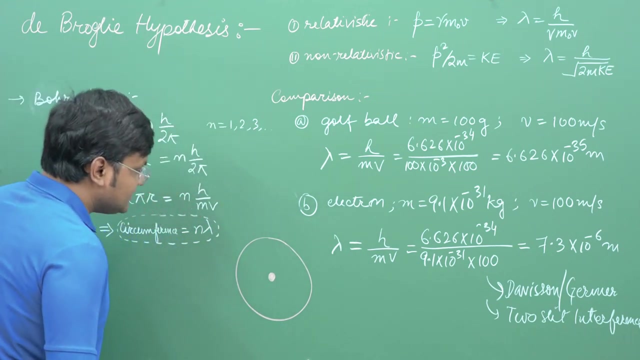 h upon mv is nothing but the de Broglie wavelength corresponding to the motion of the electron. so the circumference is actually equal to n times lambda, where n has values of 1, 2, 3 and on and on. what does this mean? it means that if we draw an electron wave in the circumference, then the 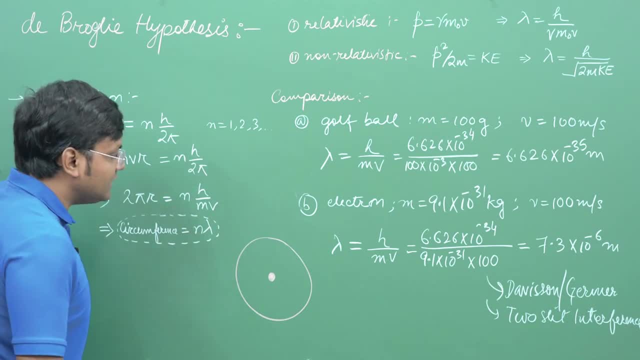 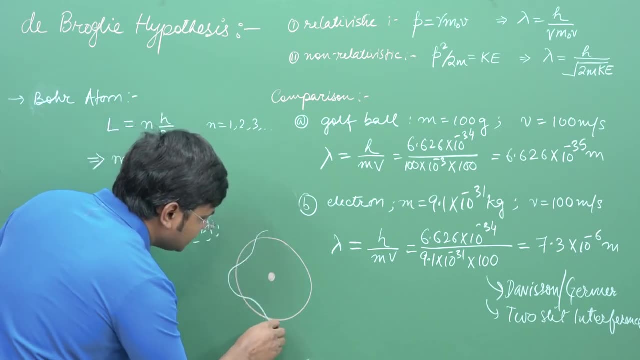 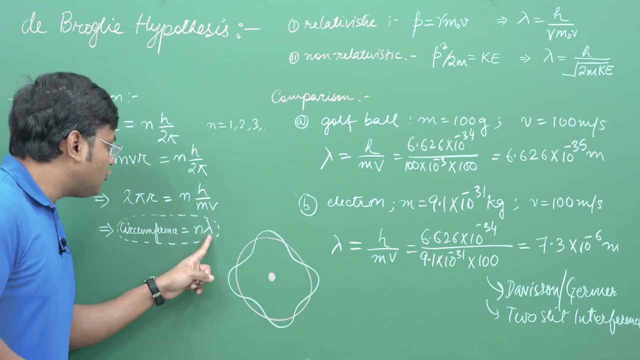 electron wave forms a standing wave pattern around the circumference, something like this. let me try to draw and do justice to a wave. yes, we are successfully able to create a fixed standing wave pattern on this circumference. so you see, if the electron has a de Broglie wave that can form a standing wave pattern at that circumference, then